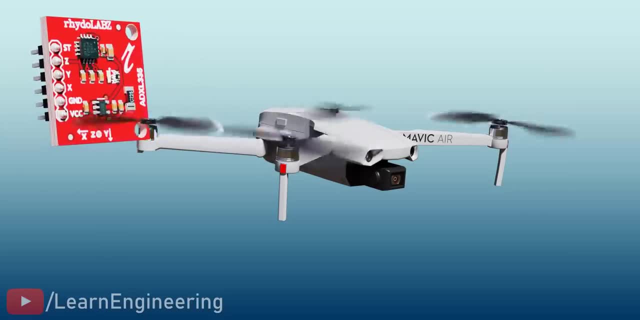 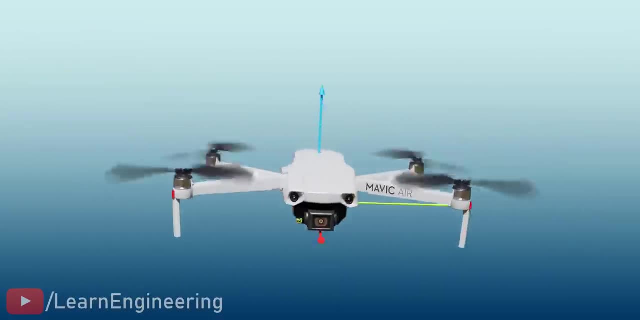 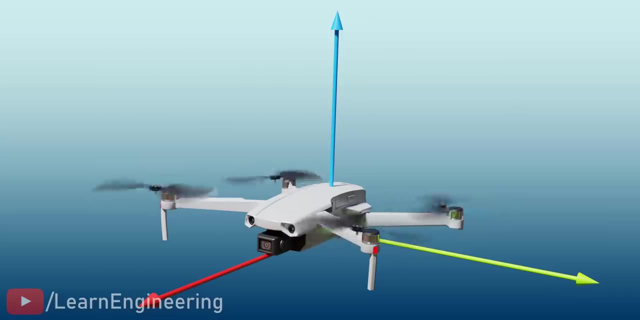 Some of them include an accelerometer, a gyroscopic sensor, flight cameras, timers and so on. The drone can achieve translational motion in three axes and it can rotate in three dimensions: roll, pitch and yaw. Let's consider the scenario of a drone hovering. 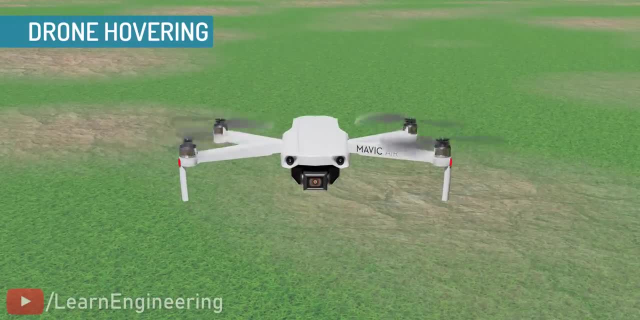 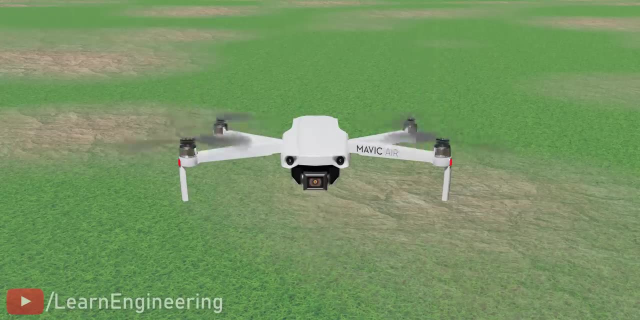 Your aim is to keep the drone hovering steadily. as shown, For a drone to hover in the air, the upward thrust must balance the downward pull of gravity. Additionally, the net torque should be zero to prevent it from spinning. That's not all The translations and angular velocities in all three directions. 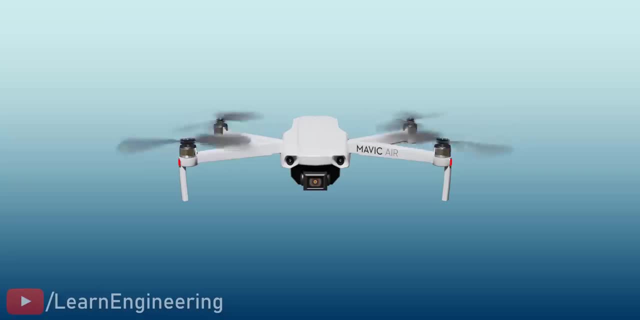 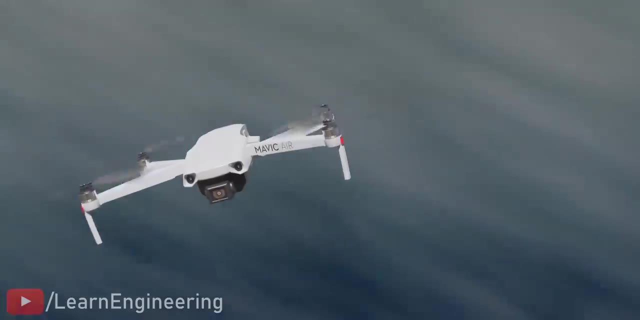 also should be zero. Let's see how the control system is applied in action. This drone was hovering in the air happily when suddenly the wind blew and the drone tilted as shown. The drone's smart controllers have to get the drone back to its normal angle. 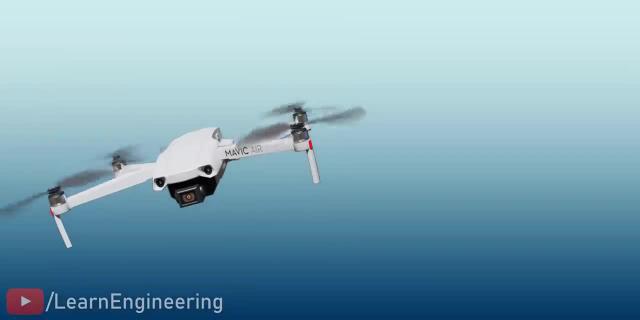 but the question is how Let's freeze the scene at a particular time when the wind is blowing. Here we're considering a change in just one angle. for simplicity of analysis. Using a few sensors, the drone can measure its speed of rotation, its direction. 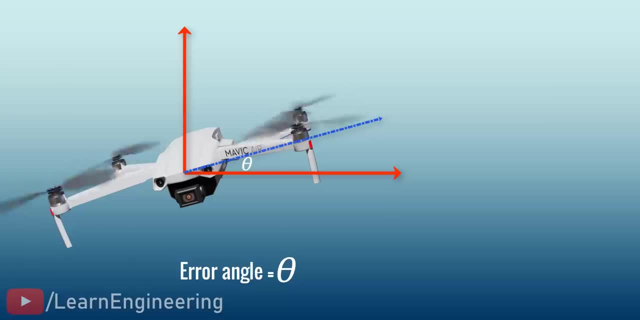 and its angle. The sensors then feed this data back to the system. The angle theta is the error with respect to the horizontal axis of the drone. In order to successfully reduce this error, the propellers should produce a torque opposite to the angle When the left and right blades spin at. 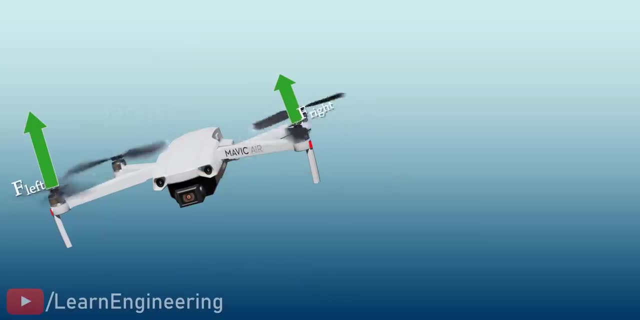 different speeds, the propellers will produce a different force and torque. The controller has to find suitable values of propeller forces throughout the restoration process. You can see that by the end of the restoration the propeller forces become equal Using a simple force analysis: the forces that the left and right propeller pairs have to produce. 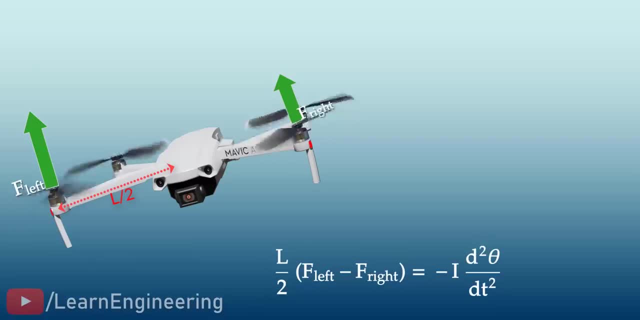 can be connected to the angle as shown. Don't worry if you can't understand all the variables in this equation. You just need to understand that the force values should vary with the error angle. However, this problem is not solved simply by making the error angle zero. 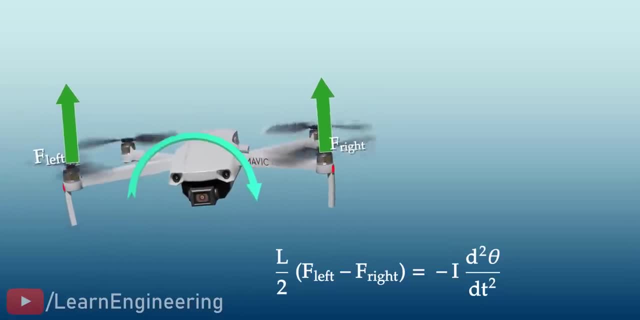 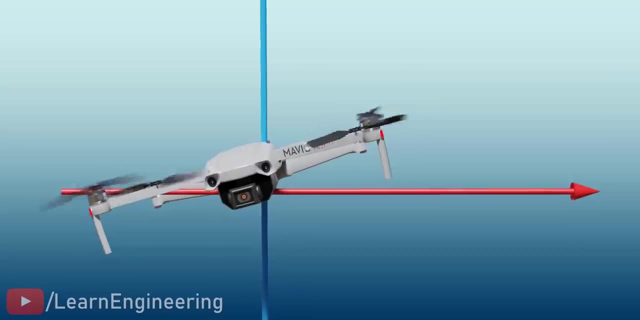 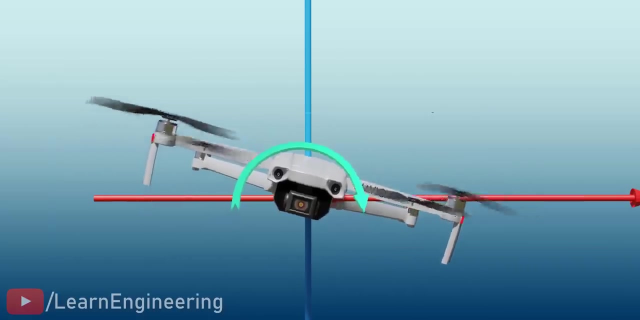 You have also to make sure that the angular velocity of the drone at zero degree is zero. If the angular velocity is not zero at the zero angle, the drone will rotate in the opposite direction, as shown. Let's plot the angular velocity that the drone has to follow in an ideal restoration process. 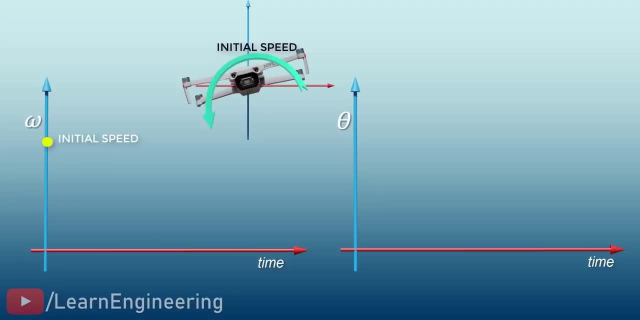 Initially, due to the wind, the drone had an angular velocity. as shown, This velocity decreases slowly due to the torque produced by the propellers. After some time, the velocity will decrease and the drone will rotate in the opposite direction. The velocity will reach zero and then go negative. 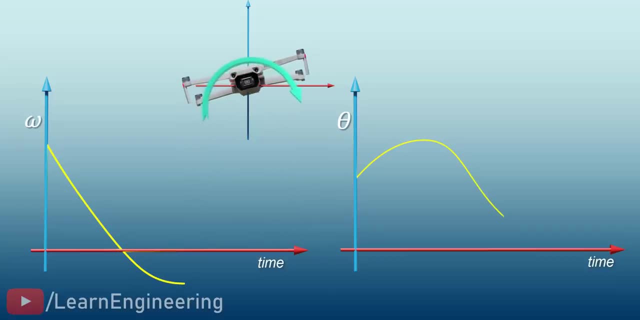 It is during this period that the drone starts to journey to a zero angle, Like we explained previously. as it approaches the zero angle, the velocity also should become zero. This means the previous force equation we derived should follow the constraint of this graph throughout the solution. This is not an easy equation to solve using calculus. 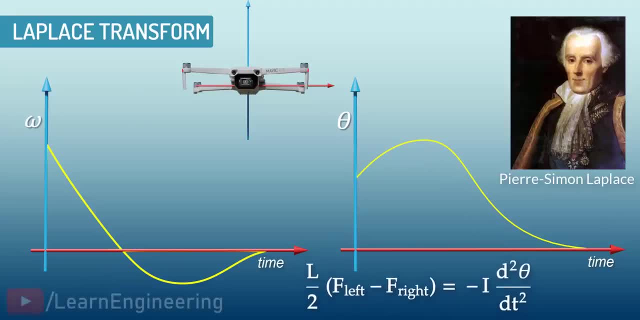 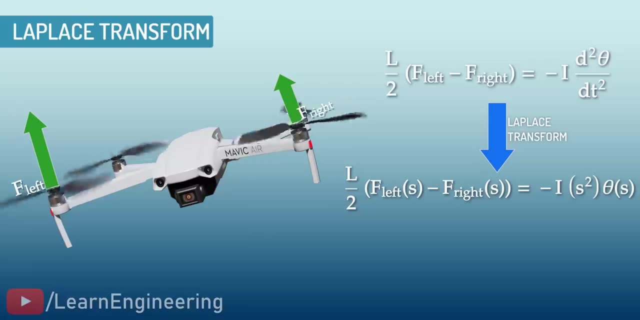 which is why Laplace transforms play a crucial role. The Laplace transform of this equation yields very simple polynomial terms, which solves the equation with ease compared to the differential equation In our case. we will be able to find out how the forces should vary with time. 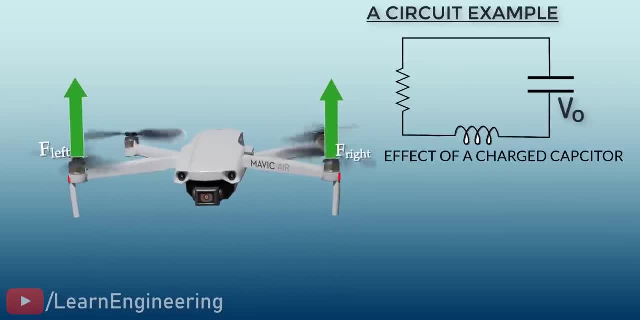 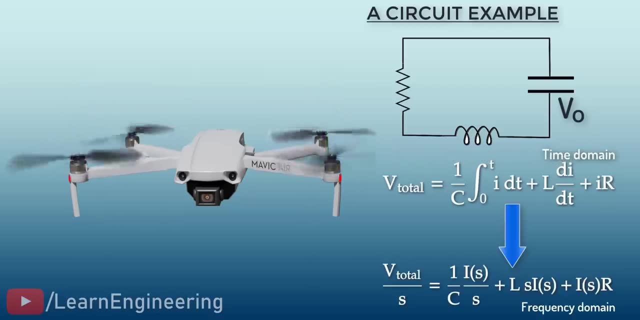 Laplace transform is a mathematical operation which converts a signal that lives in the time domain to the frequency domain. It provides us with a view of the system's reactions to input signals at different frequencies. Think of it as looking at the entire electromagnetic spectrum to gain more information about a galaxy instead of only using visible light. 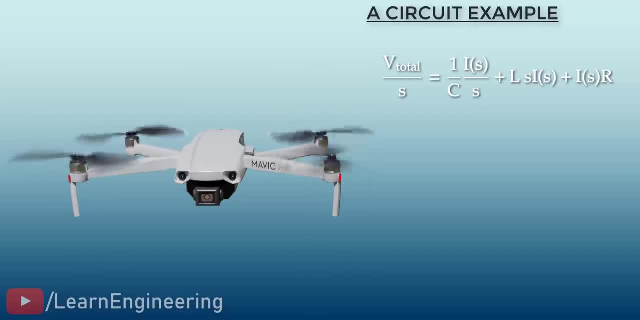 Since Laplace transform produces algebraic equations, they can be solved quite easily. To get the final output. what you have to do is just take the inverse Laplace transform of this solution. Coming back to our drone, during the disturbances, usually all the three angles will be. 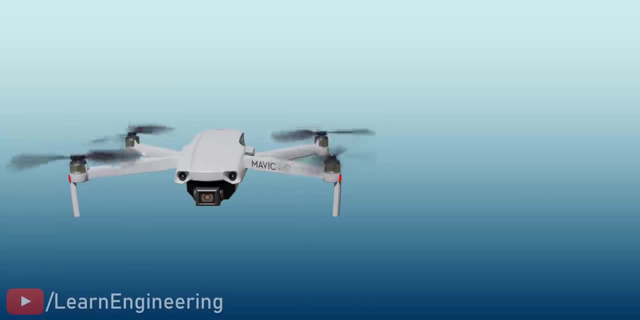 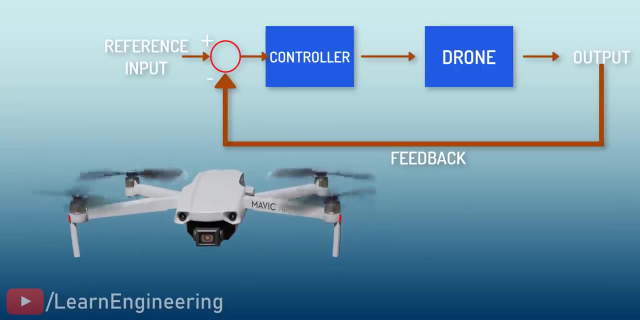 different. The sensors will constantly monitor the position of the drone and feed it back multiple times per second. Every cycle further reduces error. Advanced control algorithms are incorporated into such systems to increase accuracy and efficiency. In this drone example, we have seen that the feedback information controls the drone's motion. This type of system is called a.